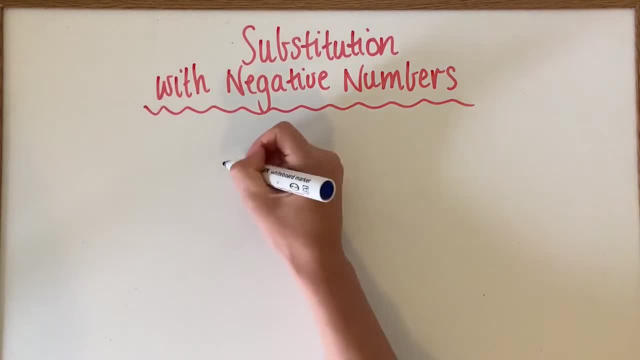 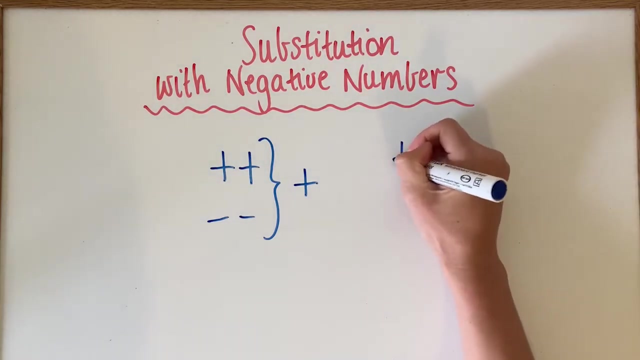 So the first thing we need to remember when we're working with negative numbers is that if you ever see two plus signs next to each other, or you see two negative signs next to each other, we can change that to just one positive sign If we see a mixture. so we see. 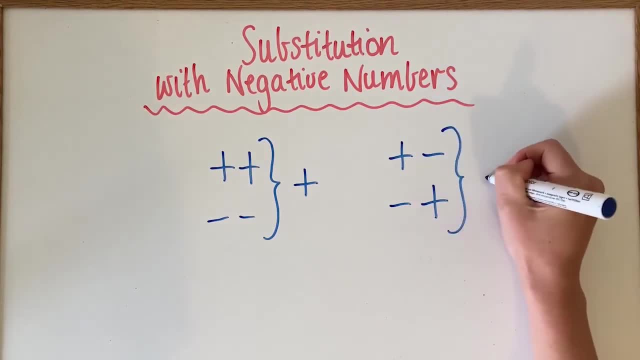 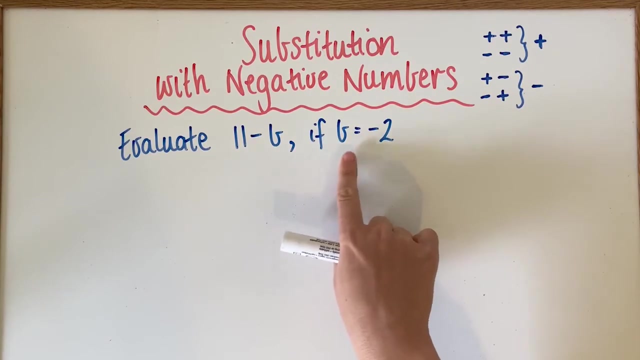 a negative and a positive, or a positive and a negative. we can change that to just a negative. It's an easy way to simplify. it makes it easier for us to understand. So that is the first thing to remember. Okay, so for this first one, we've got 11 minus b, but we're told that b is negative. 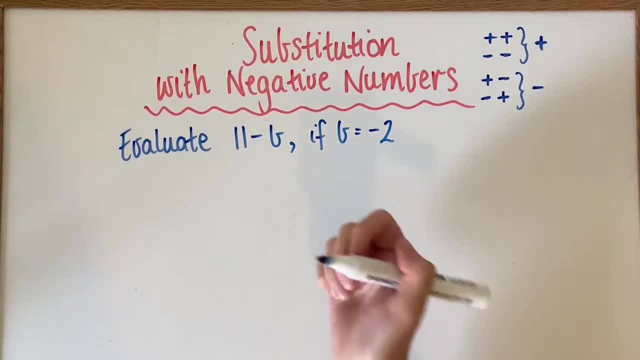 two. So we just do it like we would: a normal substitution. So we're going to go 11, take away, and then we're going to write in the minus two: Okay, so this take away stays and this one gets added in there. Okay, Now, as I said, if you have two, 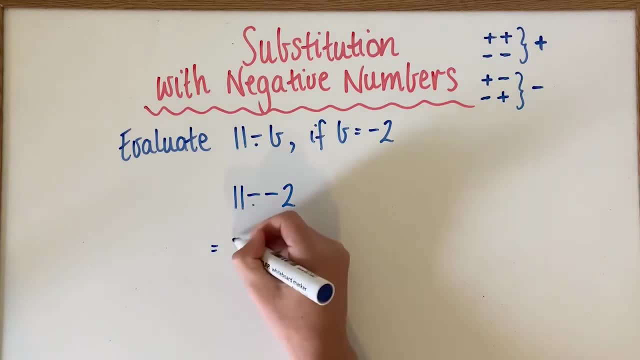 negative signs next to each other. you can convert that to a positive, So this would become 11 plus two, and then 11 plus two is going to give us 13.. So it's really important that we make sure that we're looking at the signs and that we're substituting inaccurately. Okay, here's another. 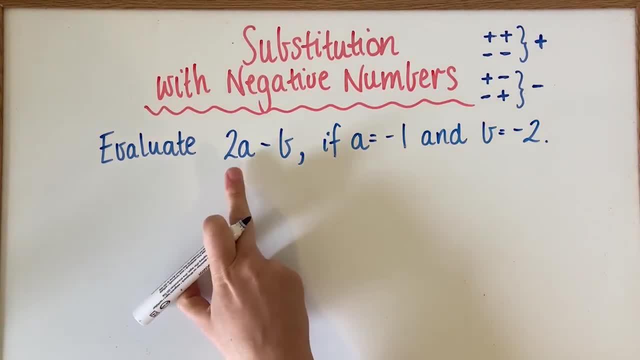 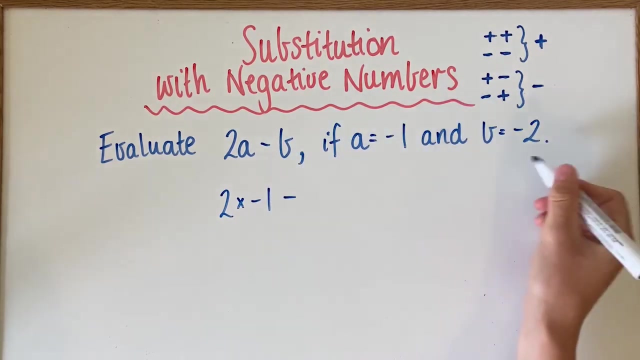 example for us. except we've got a multiplication in this one, because 2a is two times a and we're told we've got: a is negative one and b is negative two. So we write out our substitution so it's going to be a times negative, one minus, and then we put in the negative two. Okay so, 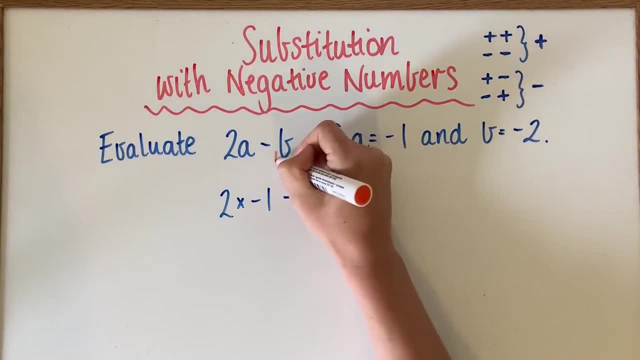 you've got to remember that this b is where this goes. Okay, so you've got to have this. negative comes down already. So we do our multiplication first, and positive and a negative, make a negative. Two times one is two. So you do the signs, first to determine what the sign is, and then you 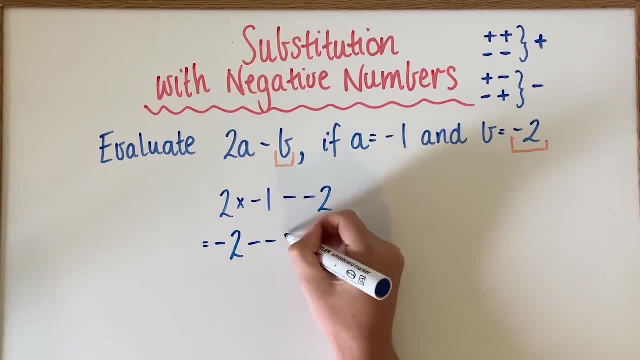 can write this like this: if we want to- again, We don't need to, but I'm going to, just so we're doing one step at a time. Then we're going to go negative two. Two negatives sitting next to each other are going to give us a positive, so it's going to be negative. two plus two, and that's.